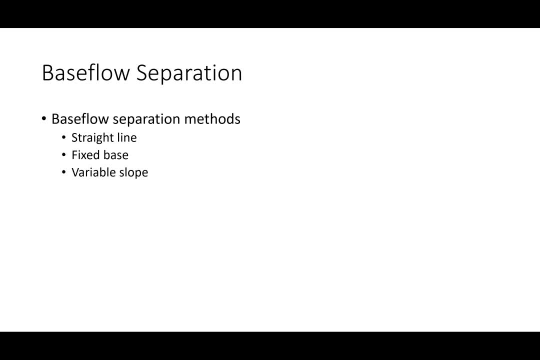 Hi everyone, welcome back. So, after long discussion about what base flow is and what contributes to base flow, and so on, Finally we are on the base flow separation methods. So there are three graphical methods that we are going to learn in this module: Straight line method, fixed base method and variable slope method. 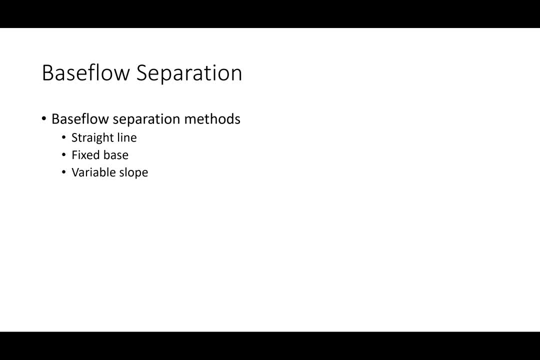 Now, these are all graphical methods. There are lots of other analytical and mathematical methods that are used in literature, and many of them are used for continuous hydrographs, But in this module we are going to stick to a single storm event and only look at these three graphical methods. 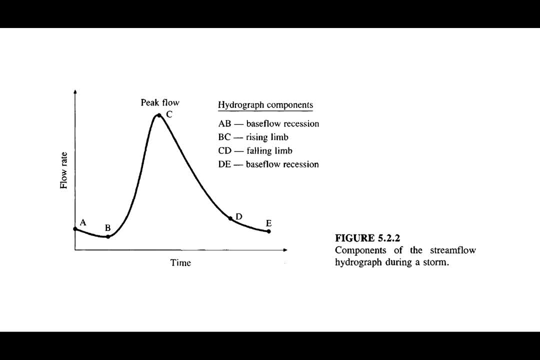 So to describe all these three methods, I will be using a plot or a hydrograph similar to what you see on the slide. This is from Chow, Maidment and May's book, figure 5.2.2.. So we have discussed before this recession curve, So this is what you see. What that means here is: from A to B: there was no direct runoff, So that was just base flow. From D to E: again the runoff stopped, So D to E is again recession. 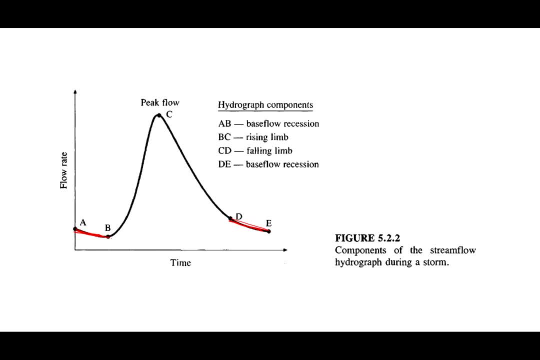 And then there is direct runoff between D and E in B and D, and our goal here is going to be looking at methods that can be used to separate the base flow from this total stream flow hydrograph. So A to B is recession, B to C is 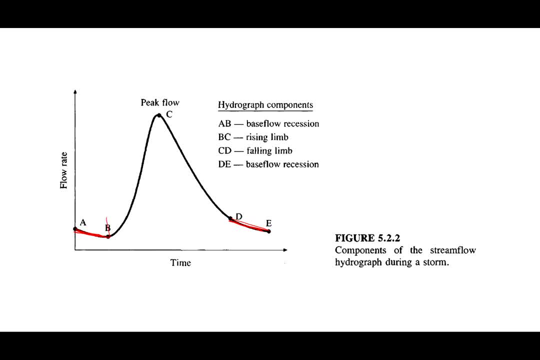 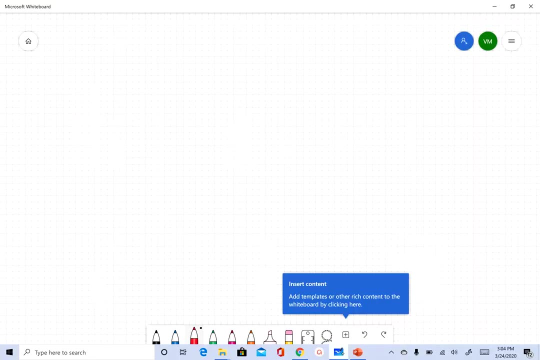 rising limb, C to D is falling limb, and D to E is again recession. So in this case we are assuming that the direction of begins at B and it ends at D. So with that, let's get started with the methods. So the first method that we are going to look at is straight line. Let me change the color. 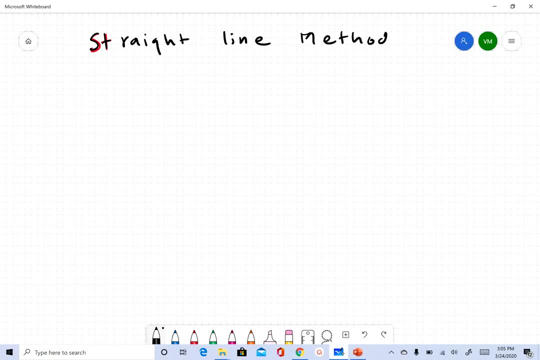 here. So I'm going to draw this hydrograph, So I'll draw the recession curve. direct runoff started and then again. So we are going to assume that this is when the direct runoff begins. I'm just going to call it A and this is when the direct runoff stopped. 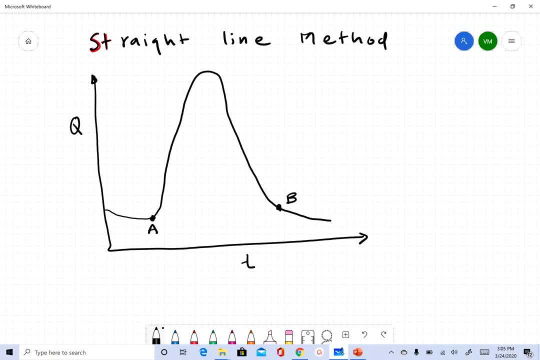 I'm going to call this B. So in straight line method, you first find out when direct runoff started and when it ended, and once you know these two points, all you do is connect A and B. So I'll just use a different color here. So you connect A and B using a straight line, and then all this area. 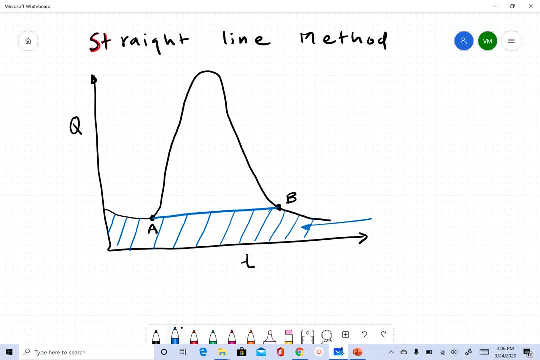 is base flow And then direct runoff, So I will just use a different color for direct runoff. So our green area is direct runoff and the blue hatched area is base flow. So the the steps for straight line method are simple. find A and B. 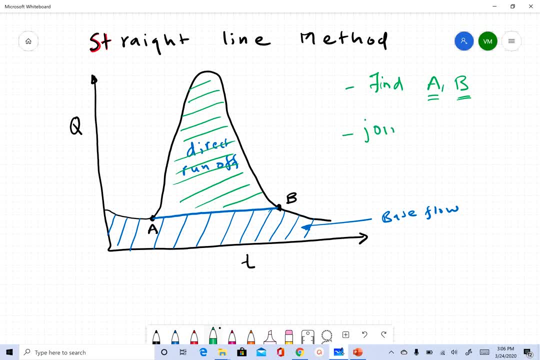 A is when the direct runoff starts, B is when the direct runoff stops, and then simply join A- B using a straight line. Now, in some books they call this this as horizontal line method, which means that you just draw a horizontal line. I'm calling this. 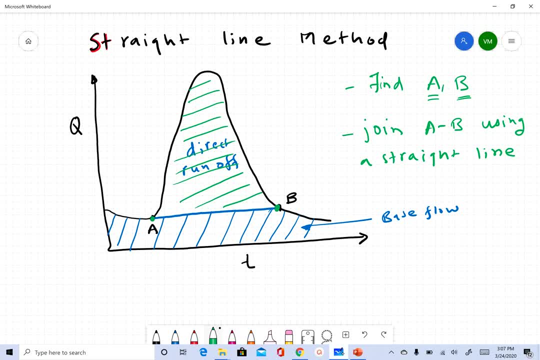 straight line because a and B may not fall on the same level. so if it is B, if B is higher or lower, you will have an inclined line. so so there are few more names that are used for straight line method. so, as I said, horizontal line method. for me horizontal line method is just a simplified 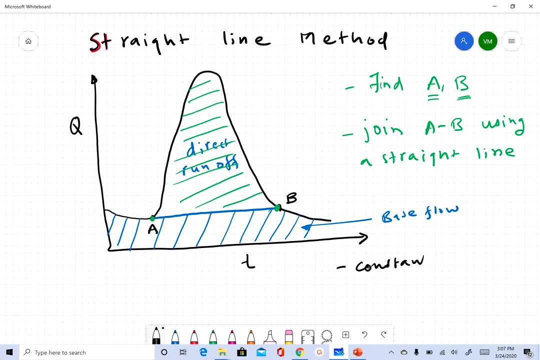 form of straight line method. some books also use constant discharge method. so again, constant discharge, meaning that this line is horizontal and the flow along that line is constant. so this is straight line method. now you may ask: how do we know points A and B with any graphical method? this is a subjective 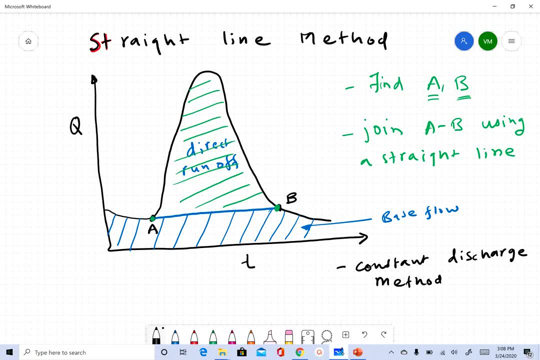 approach. it means the the final answer that you get depends on where you define your point: A and B. okay, so we don't need to worry at this point. how do we find A and B when we have actual data? but this comes through practice and experience, so that's straight line method. 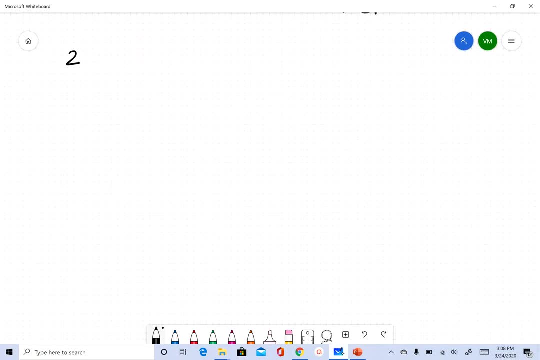 that was our first method. the second method that we are going to look at is fixed base method. I will again draw this line, this hydrograph here, plus or minus 2, and so this is señalThen I will draw three lines that I call it or trade a triangle. I will also draw all starting keys for our circuit. the fermo and the arrow keys are 0.0 and 5 and 1, which tells us that the fit-back line method isестеjm peine. I will also draw three lines that are tilde and 1, which tells me that the use of a identical Tal continuously affects the ability to drug. why do jobs這個? 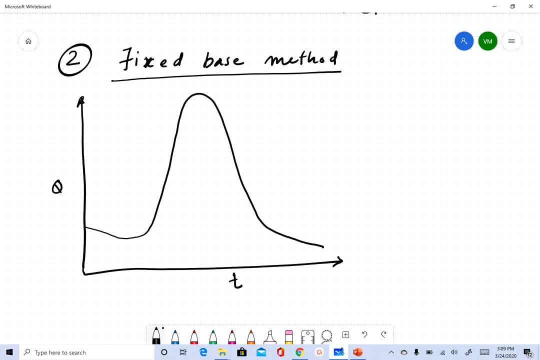 so in fixed base method you need to find your point a, so find a. so a is again when the direct runoff begins, and this is our Q peak, okay, so I'll just draw a dash line here. and this method assumes that the direct runoff will end after time n after the peak. so I'm just going to. 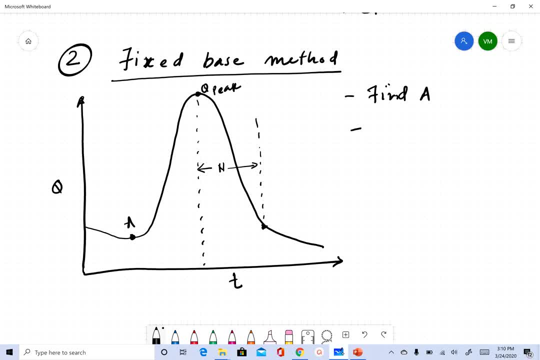 you draw that here. so runoff ends or direct runoff ends and days after Q peak- okay, so once you, that will give us point B. okay now, what you do to get the base flow is you extend this recession curve before runoff forward until Q peak. so I'm going to use blue color here. okay, so I just used the slope of the pre event curve, recession curve. prove recession curve. so I will stick to this here also until Q peak, mid- chore curve leads to recession curve. fore in Q peak mode: okay, great, f the curve weaving and see what happens after F, go to the возcupert method. okay, let's just call it recession curve. before runoff forward. so this is a pre event curve. so f and gi, it's just the different top and bottom move before f and gi. it's just the different top and bottom move after f and gi, it's just the different top and bottom move, the recession curve and that second curve, these appropriate pre event curve, the pas barnard o. 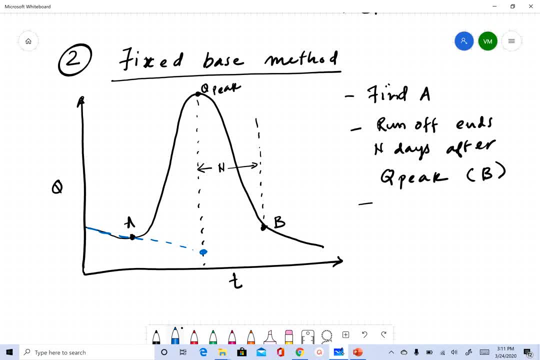 so we have the presum encarale vezmar 000 Только this curve when the recession curve ends, to extrapolate it until I reach the time to peak. so extrapolate, prevent flow until Q, P, okay, and then you connect this point. so let's call this point as C. 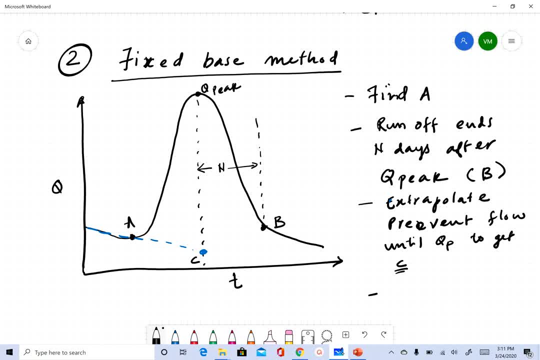 until Q P to get C- okay, and then just connect C and B. or we can say Q P to get C- okay, and then you connect this point. so let's call this point as C until Q P to get C- okay, and then just connect C and B. or we can say: connect C and B. or we can say Q P to get C- okay, and then just connect C and B. or we can say Q P to get C- okay, and then just connect C and B. or we can say Q P to get C- okay, and then just connect C and B. or we can say: 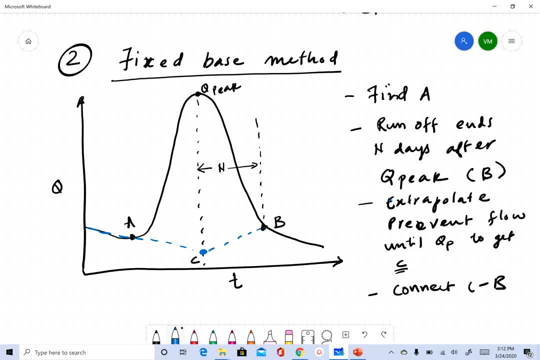 connect, yeah, C and B, so use so. once you connect, yeah, C and B, so use so. once you connect, yeah, C and B, so use so. once you do that. this is our base flow in blue. do that. this is our base flow in blue. do that: this is our base flow in blue hashed area and the green is our direct 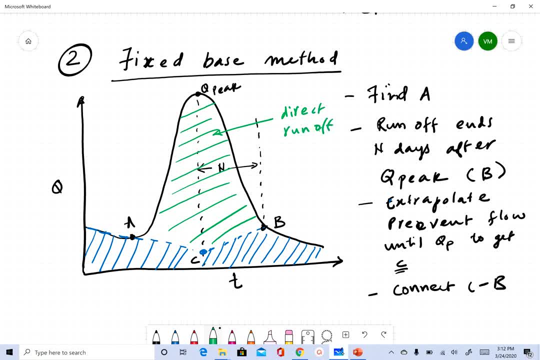 hashed area and the green is our direct hashed area and the green is our direct runoff, runoff, runoff, and that's our base floor. okay, so the, the and that's our base floor. okay. so the, the, and that's our base floor. okay, so the. the extrapolation of pre-event flow until: 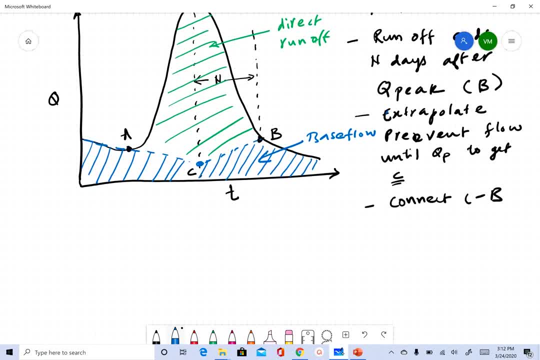 extrapolation of pre-event flow until extrapolation of pre-event flow until point C, which is our Q peak, is easy. you point C, which is our Q peak, is easy. you point C, which is our Q peak, is easy. you may then wonder: so how do we know what? 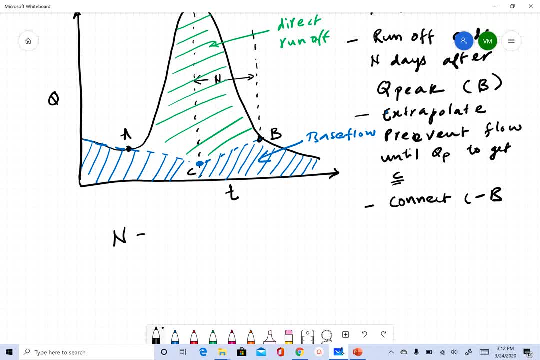 may then wonder: so how do we know what? may then wonder: so how do we know what? n is this? there is an empirical formula. n is this: there is an empirical formula. n is this: there is an empirical formula that you can use to find n, so that 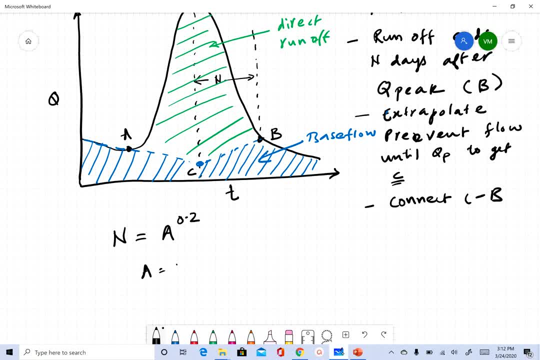 that you can use to find n. so that that you can use to find n, so that empirical formula. empirical formula. empirical formula is: n equals to a to the power of 0.2, is n equals to a to the power of 0.2, is n equals to a to the power of 0.2, and a is the watershed area in square. 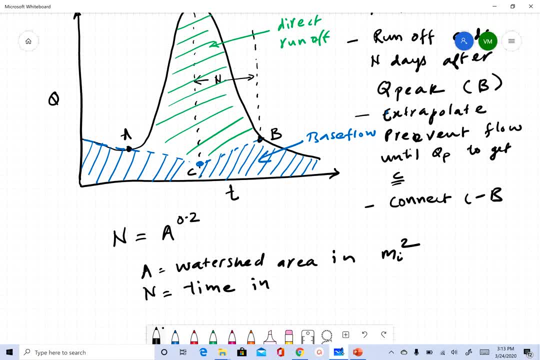 and a is the watershed area in square and a is the watershed area in square miles, and n is in days, so time in days miles. and n is in days, so time in days miles. and n is in days, so time in days, okay, and I have used this expression n. 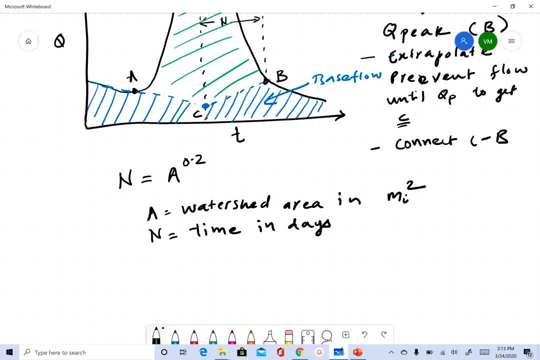 okay, and I have used this expression: n. okay, and I have used this expression: n equal to a to the power of 0.2, and equal to a to the power of 0.2, and equal to a to the power of 0.2. and just to give you an idea for area of 100. 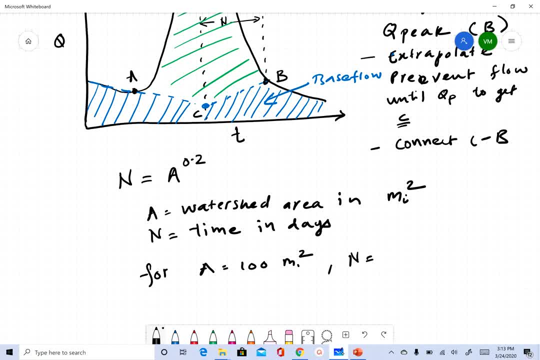 just to give you an idea for area of 100. just to give you an idea for area of 100 square miles. you get n equal to 60 square miles. you get n equal to 60 square miles. you get n equal to 60, something around 60 hours. so I converted. 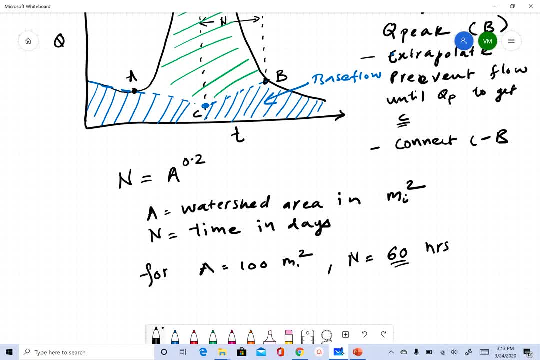 something around 60 hours. so I converted something around 60 hours. so I converted the answer that you get in days to hours, the answer that you get in days to hours, the answer that you get in days to hours, and you get something around 60 hours. 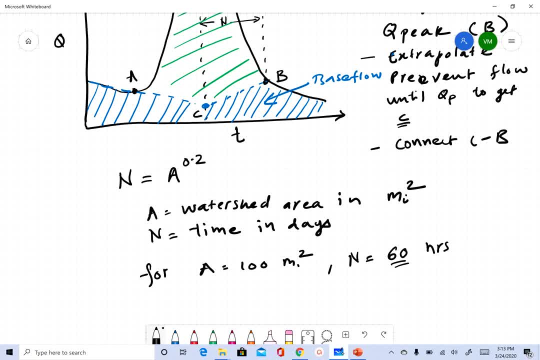 and you get something around 60 hours. and you get something around 60 hours which for me seems too long. so the which for me seems too long, so the which for me seems too long, so the, the literature says that you should. the literature says that you should. 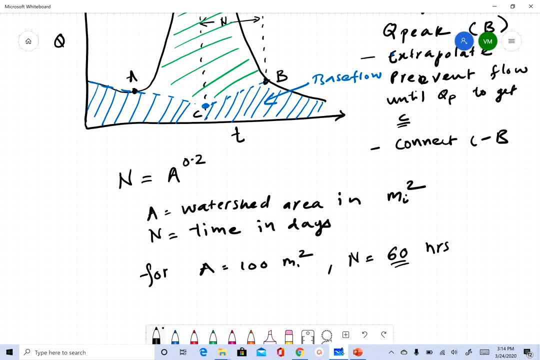 the literature says that you should. usually this n equals to a to the power. usually this n equals to a to the power. usually this n equals to a to the power of 0.2 works for large watersheds, so we. of 0.2 works for large watersheds, so we. 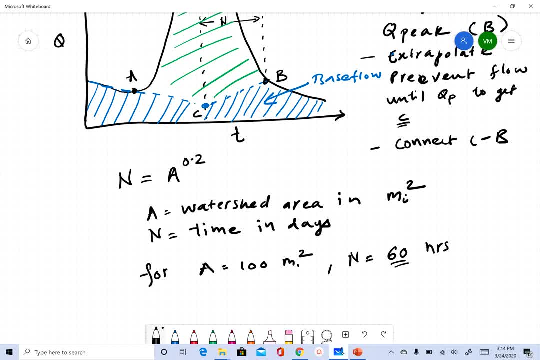 of 0.2 works for large watersheds. so we have used this area of 100 square miles, have used this area of 100 square miles, have used this area of 100 square miles in many of our heck HMS labs and you see, in many of our heck HMS labs, and you see. 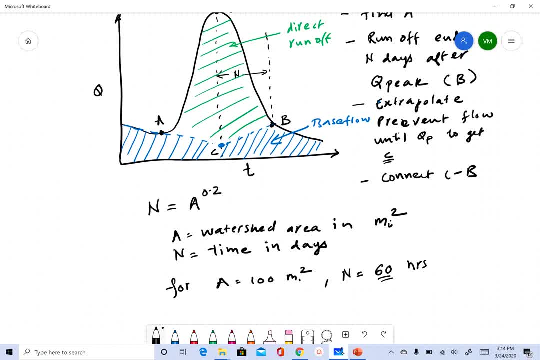 in many of our heck HMS labs and you see that most of the times the hydrograph that most of the times the hydrograph that, most of the times the hydrograph doesn't even last for 60 hours, so the doesn't even last for 60 hours. so the 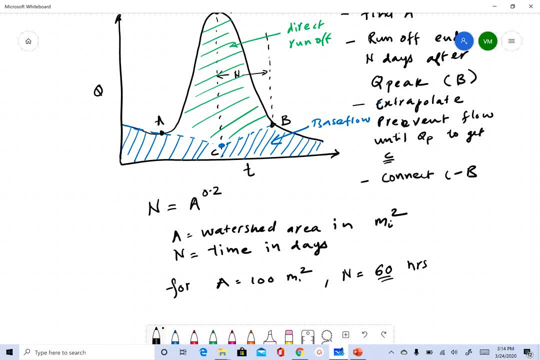 doesn't even last for 60 hours. so the the fact that this n after peak is equal, the fact that this n after peak is equal to 60 hours, and that's when the runoff to 60 hours and that's when the runoff to 60 hours and that's when the runoff start, doesn't make sense for for this. 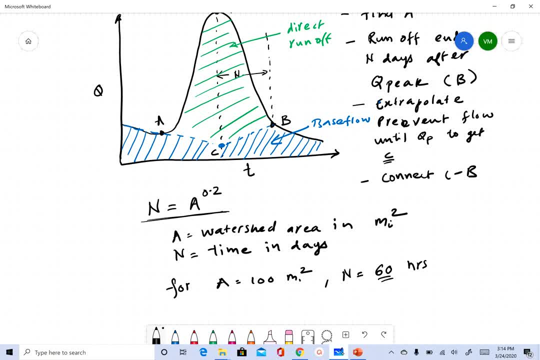 start doesn't make sense for for this start doesn't make sense for for this small area, but anyway, this is what is small area, but anyway, this is what is small area, but anyway, this is what is available and some people use it, so this available and some people use it, so this. 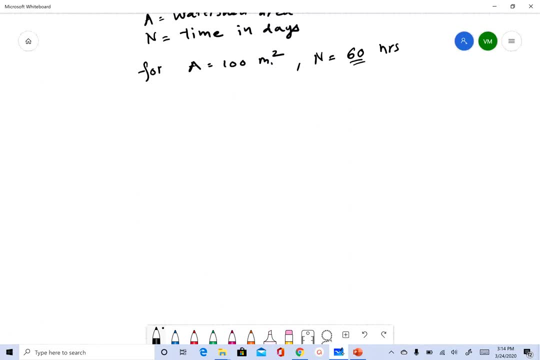 available and some people use it. so this is how you can get this n to get the is how you can get this n to get the is how you can get this n to get the point B. so that's our fixed base method. point B- so that's our fixed base method. 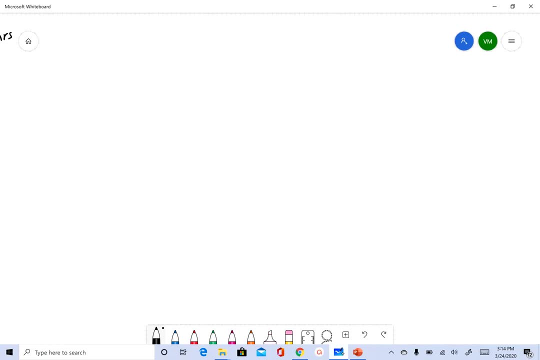 point B. so that's our fixed base method. the third method is called variable. the third method is called variable. the third method is called variable slope method. slope method, slope method. I will again draw my hydrograph here. okay, okay, okay, so we'll, so, we'll, so, we'll fix that. 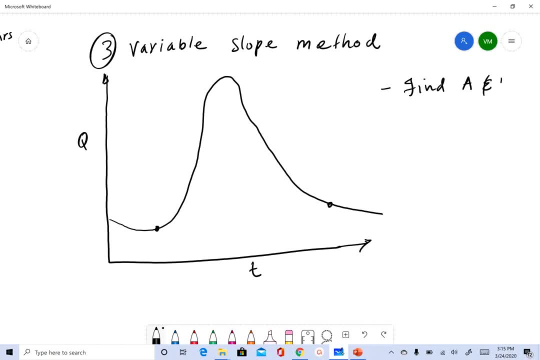 fix that. fix that here, fix that here. find point a and point b. find a and b. so a is when the direct runoff will start, b is when the direct runoff will stop. and finding a and b is again subjective, so we will use our own judgment to find where point a and b is. so this is our cube peak. 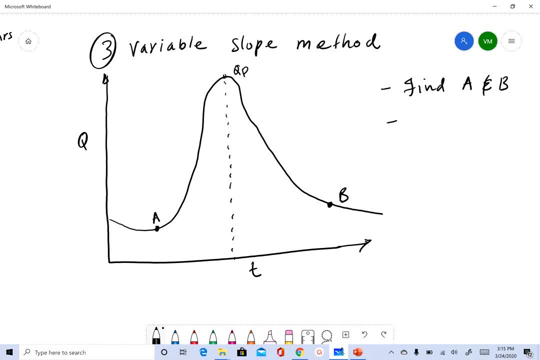 so, after you point a and b, then you the first step or the second step. in this case is similar to what we did for fixed base method. so extrapolate, prevent flow until q peak to get point c. so i will do that. so i'm going to extrapolate this until i get this point, which is c. 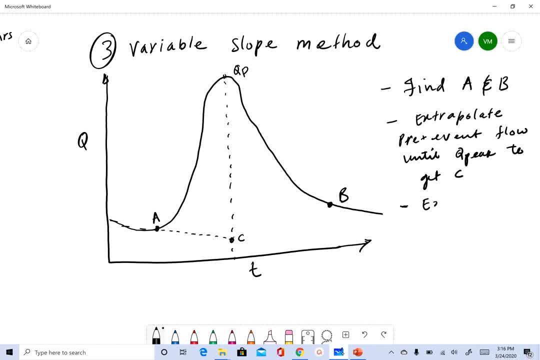 now the next step is you extrapolate the post event flow, post event flow backward until inflection point. so, if you remember from the last clip, inflection point is when you will see a change in slope on the recession limb. so on this plot maybe you can see. and again, i did this on purpose, so let's assume. 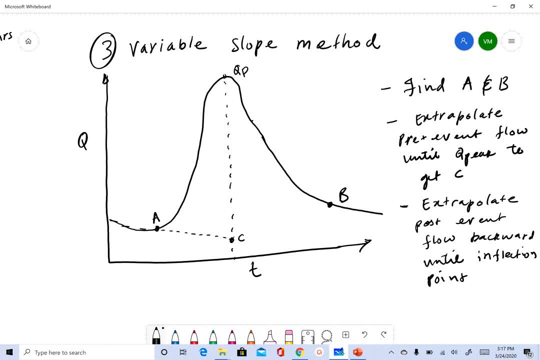 this is our inflection point, which is our- or maybe let's do it somewhere here. okay, so let's assume this is our inflection point and I'll talk about how to get that inflection point once I'm done with this inflection point D. okay, so this is my inflection point here. so 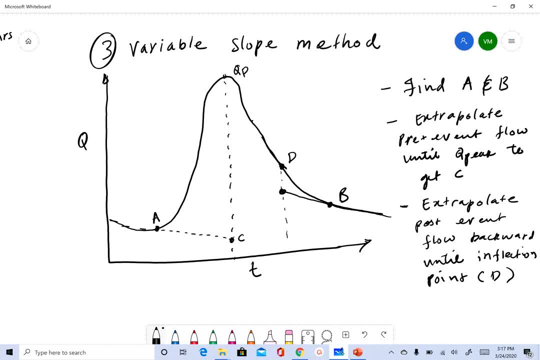 I'm going to extrapolate my post event flow backward like this: until I hit, until I get my. so maybe this is my inflection point and then this is my point D, okay. so once you get that point D, then you connect C and D, okay so? 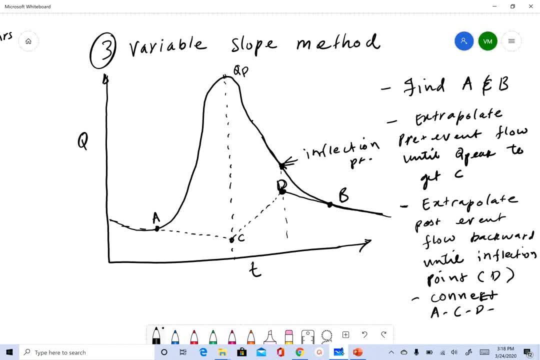 connect A, C, B and B. so we connected all this and then, once you do that, this is our base flow. okay, so this is base flow, and then this is our direct runoff. okay, so this is base flow, and then this is our direct runoff. so let me repeat the steps. so the first step was to find A and B. so A is when the 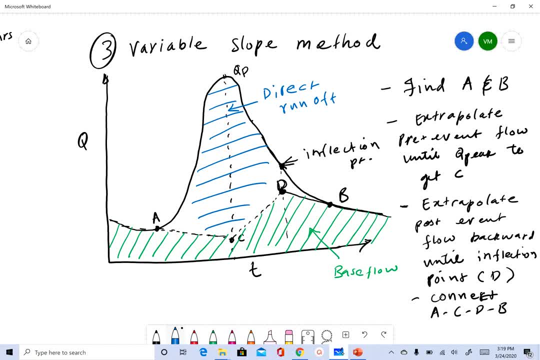 direct runoff starts, B is when the direct runoff stops. finding this point is subjective, so we will use our judgment to locate those points. once you do that, you extrapolate the pre event flow until the time to peak to get C, C, and then the next step is to find the inflection point. and once you find the, 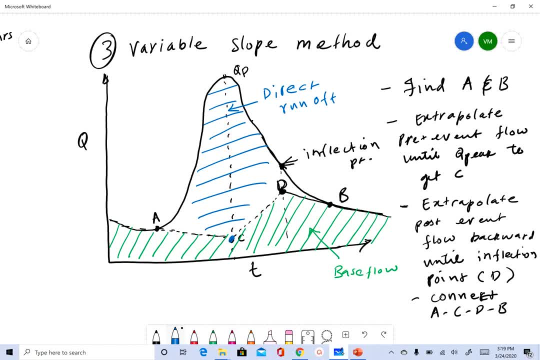 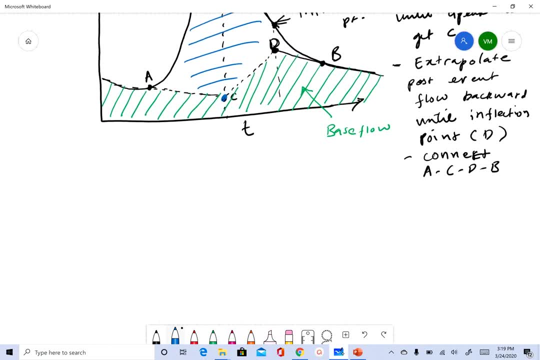 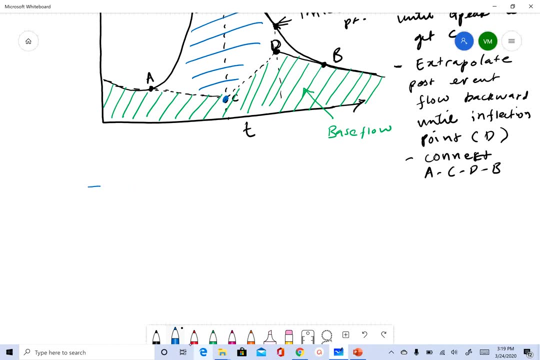 inflection point, you extrapolate the post event flow backward until you hit the inflection point to gate D and then you just connect all those points to to get the base flow. now you may ask how do we get inflection point if you really want to do it mathematically? so at inflection point. 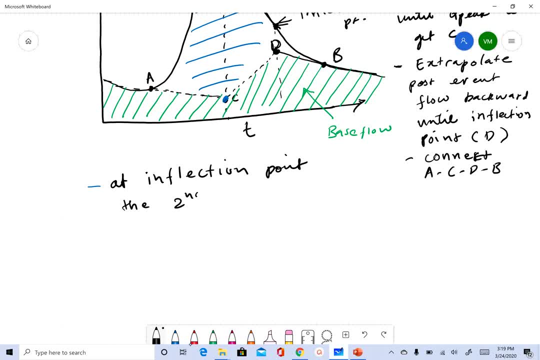 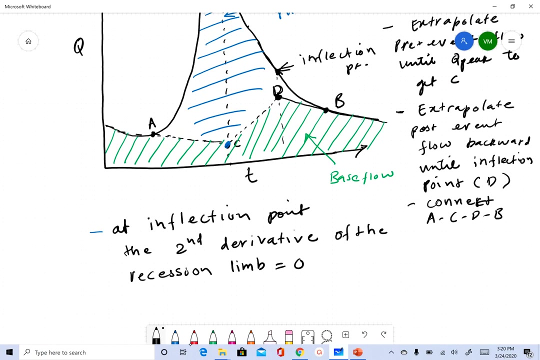 the second derivative of the recession curve is zero. the recession limb is equal to zero. so that will be the mathematical. we are finding the inflection point. if you don't know the inflection point, you can just use the non-physical derivative as theazuge or the. 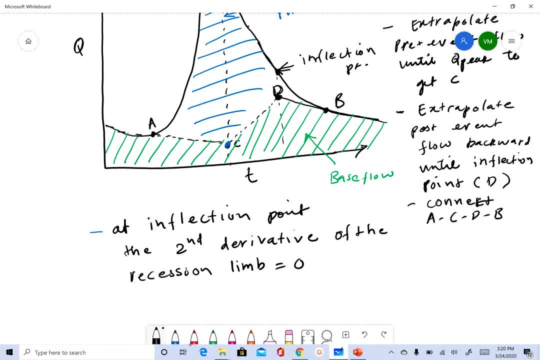 unphysical derivative. and if you don't want to do that, you can use your you or you can eyeball and see where the the slope of this line changes and you just mark that as inflection point in this class. I'm not going to make it hard for 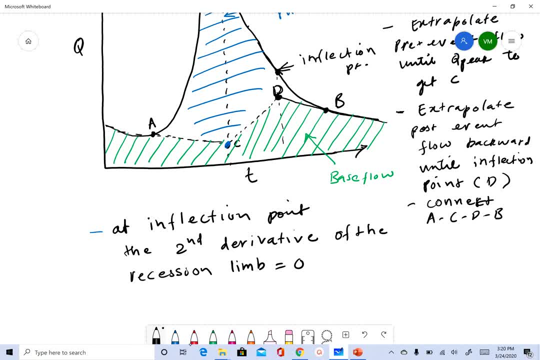 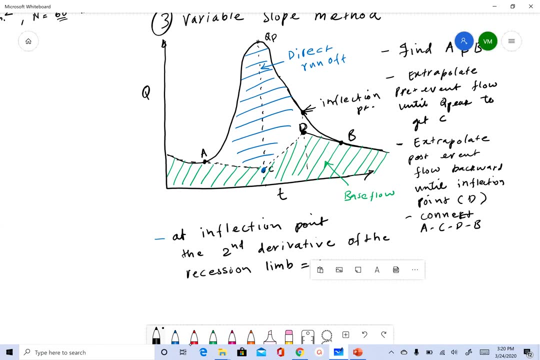 you when we do an assignment. I'm just going to give you where the inflection point is, but for your homework, if you want, you can do some calculations and find the secondary with you and wherever it becomes, you mark that as inflection point. so this is the variable slope method. so, as you saw, we looked at. 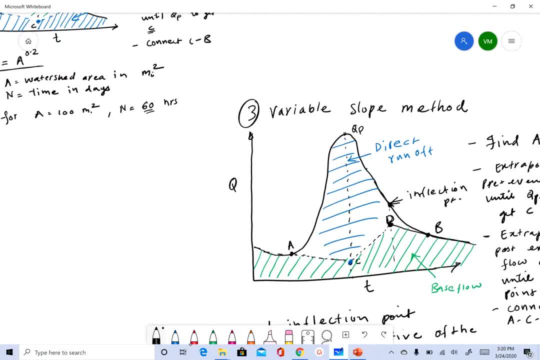 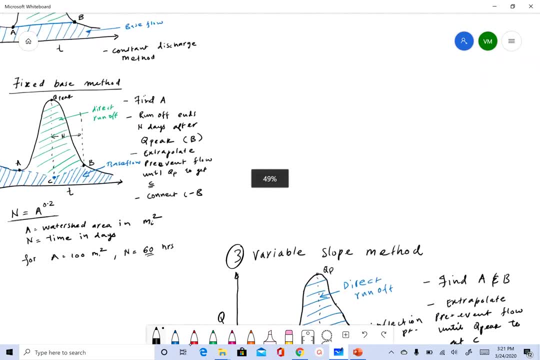 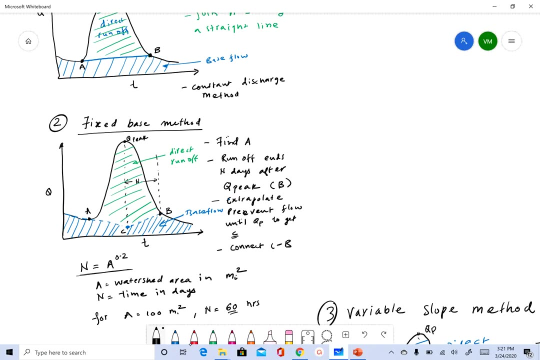 constant discharge. now i'm calling it so: straight line method, fixed base method and variable slope method. you may ask which method should i use? so the answer is: it depends on how your stream flow hydrograph looks like and what you are comfortable with. so, and these are: 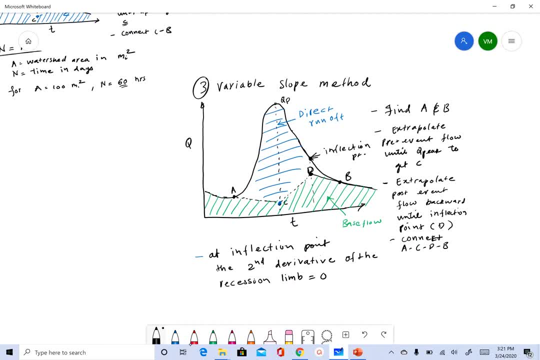 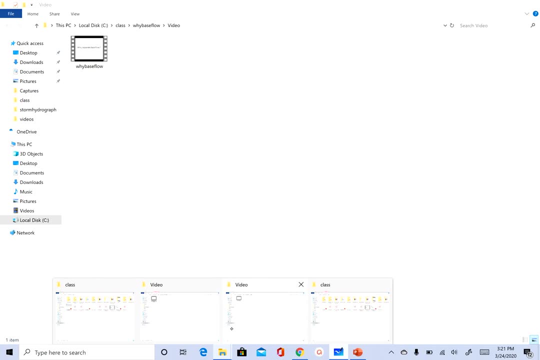 all subjective methods. so if i have to recommend you, i would either use the fixed base method or variable slope method, and variable slope method looks more reasonable to me and it looks more like that- that recession curve that we looked at. so if you are comfortable with that, you can. 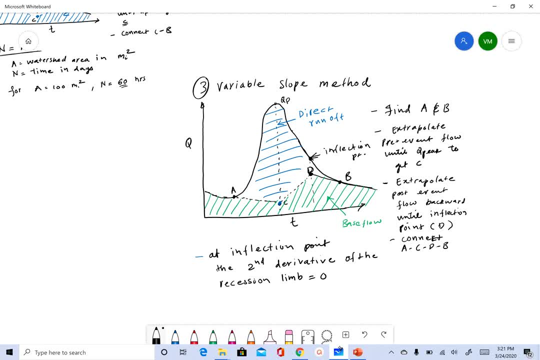 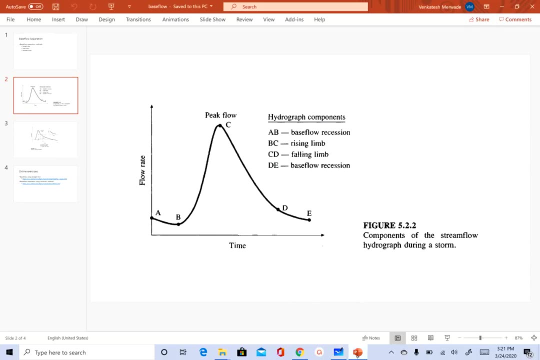 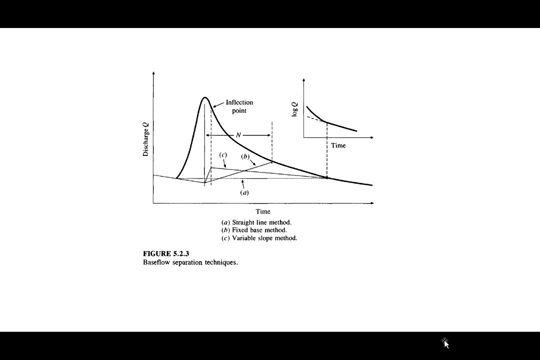 use the fixed base method or, if you are comfortable with that, you can use the variable slope method. so if i have to, if i have to draw a curve, this looks similar to what what i draw before in one of my previous clips, so variable slope method would be my preferable method. so let's go back. 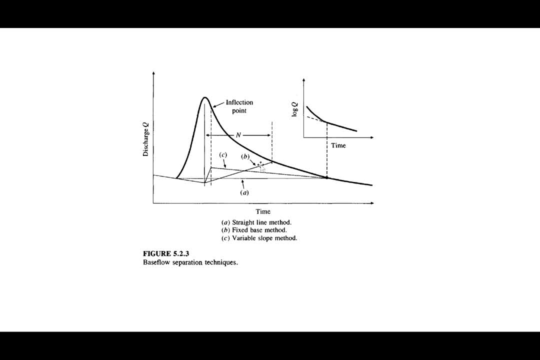 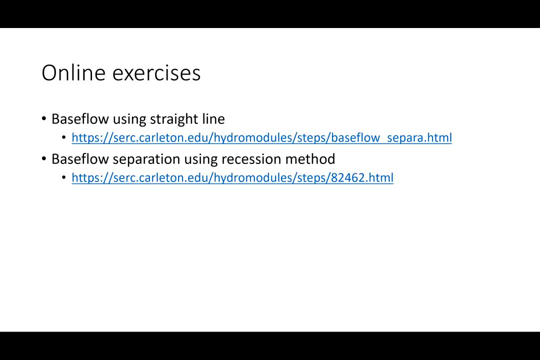 to our powerpoint slide and i'm going to show you all these three methods. so this figure is again from chao mademont and may's figure 5.2.3. and and finally, i'm giving you two links here. so these links talk. 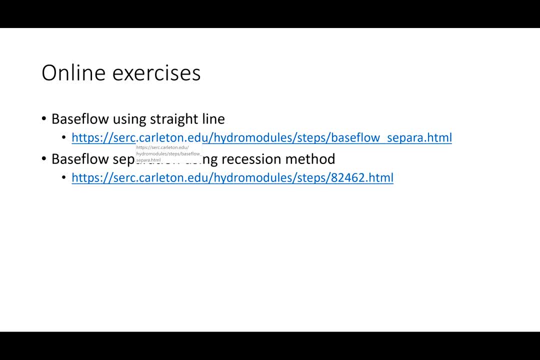 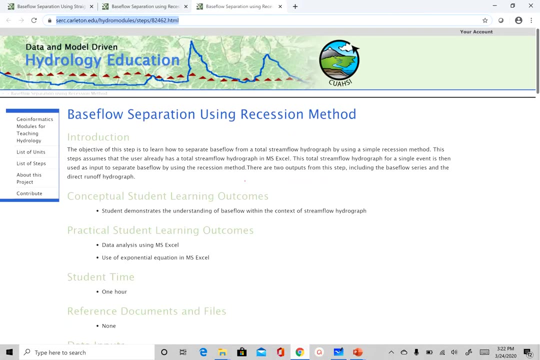 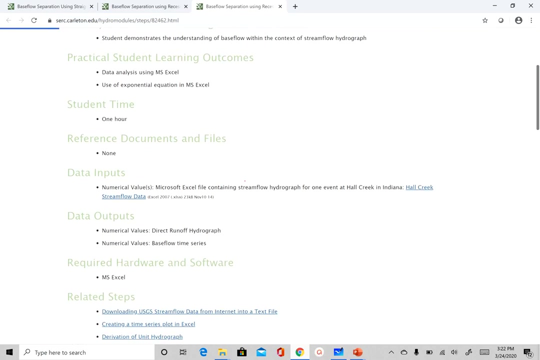 about using the. the first link talks about using straight line method on an actual storm event and the second link talks about how to use the recession method. so this is a method that is not a graphical method, and this is the method that is used in heckhms, so if i click on that, so this is how the online module looks like and, again, this is. 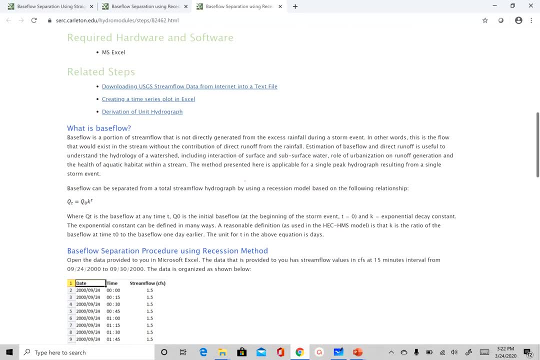 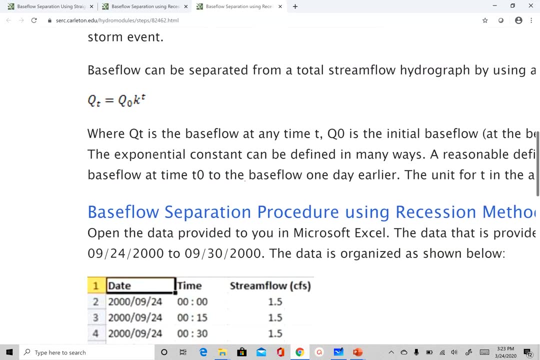 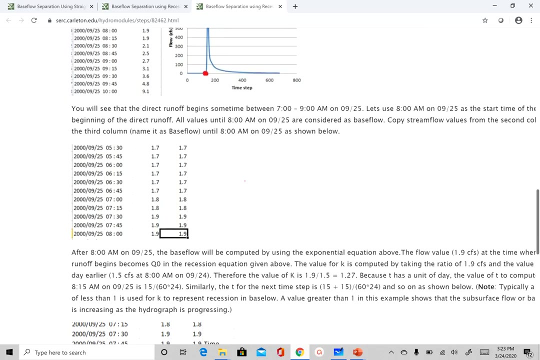 something that i developed as a part of a project. so this module takes you through different steps on how to get the data, and so this is the guess- i cannot use the pen- that that the HEC-HMS model uses for recession curve, and then this model. 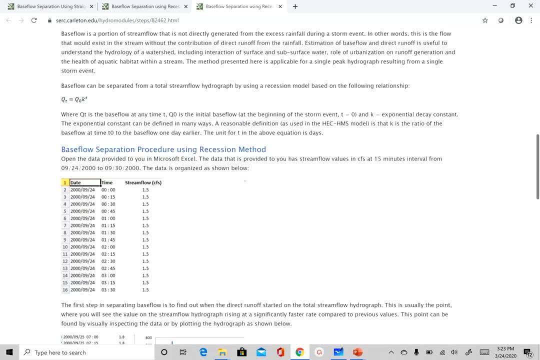 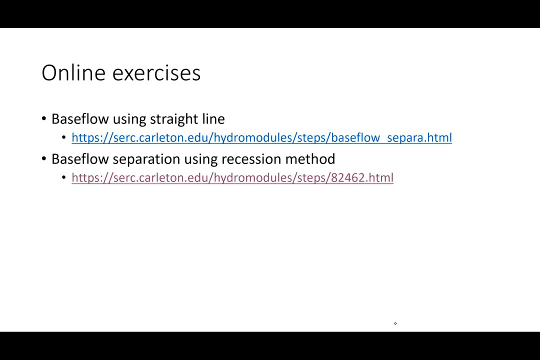 walks you through the different steps to to get the base flow using that method, and we will be using this in in our next HEC-HMS labs too. so with that I'll stop here, and in the next video we will do a small assignment on how to actually use. 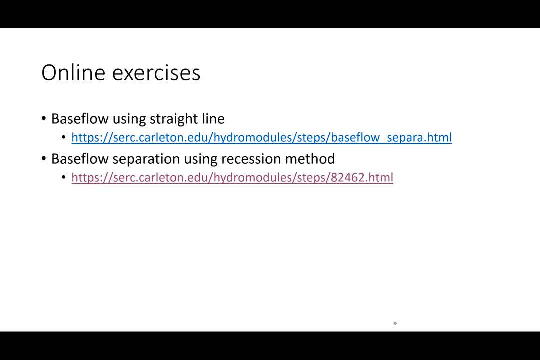 these methods on a hydrograph. so with that, I hope you enjoyed this video and I will see you soon. if you have any questions, feel free to email me, and until then, goodbye.